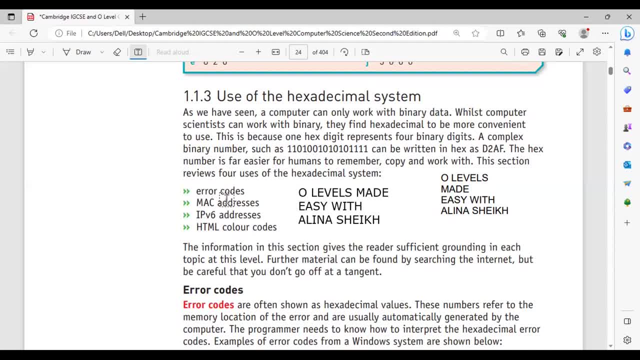 Now we have four users of hexadecimal error codes, MAC address, IPv6, HTML codes. so we will read this today. the information is here. it gives us sufficient grounding. if we want more information, then we can take it from the internet. 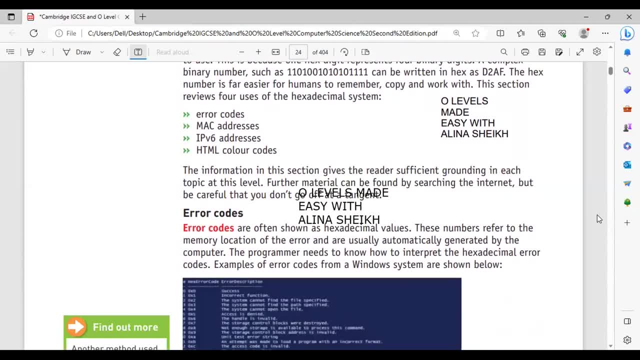 First of all we come to the error codes. what are the error codes? when there is a problem in the computer, then the computer automatically generates an error that this error has occurred, and that error code is shown in hexadecimal values. The work is done by the computer in its binary. it converts it in front of us and shows that this problem has come in hexadecimal. this problem has come, so the programmer should at least know hexadecimal that he interprets what the error is. 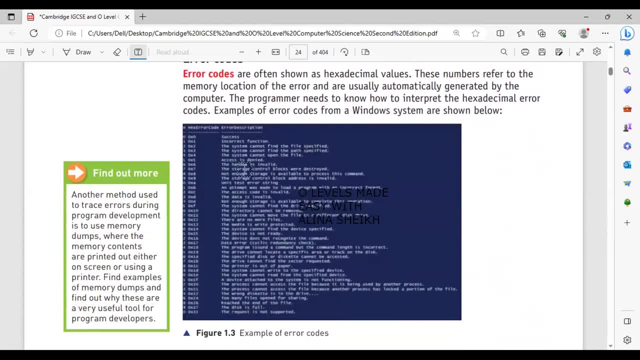 Now here we see another method used to trace errors during program development. that is, if there is a problem in the program development, then the memory is dumped. what happens in it is that the contents, whatever the problem is, whatever the content of the memory is, it is printed. if there is a problem in it, then hexadecimal. they know that, the programmers know it. they solve it through it. we will see it in a little more detail. 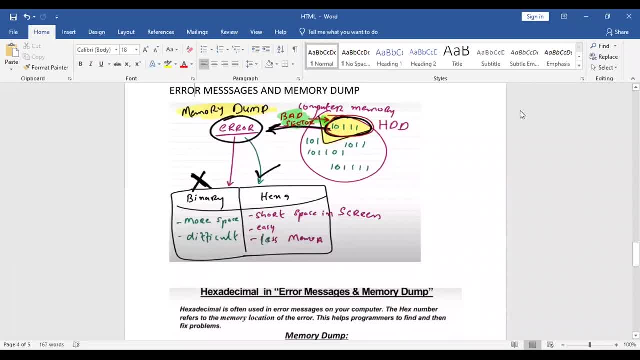 Here I have explained to you through a diagram. now see, the memory is dumped. what is dumped? when we dump garbage, then it becomes garbage. bad sector here. I have represented it in the same way. it is HDD, where all the memory of the computer is stored. there is a bad sector here. that is, there is a problem here. there is a problem on it. call it a bad sector, call it an error, call it a memory dump. 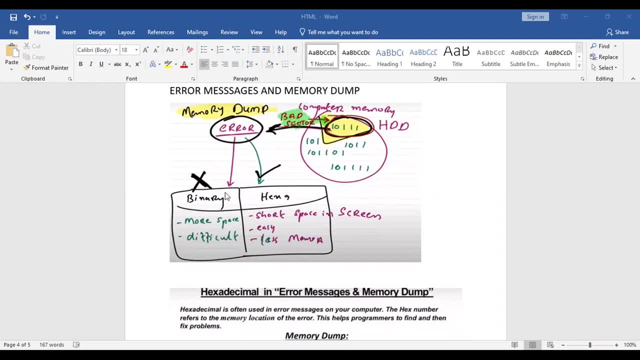 Now this error. this computer can tell us in binary, but we have kept an option on it: It is not binary, we need hexadecimal. why hexadecimal? if so many ones have come, then it will be difficult for us and we want to make the work easy. so we told the computer that the problem that is coming to us you tell us in hexadecimal. so the problem of this bad sector, it has represented us in hexadecimal. short space and screen is easy and takes less memory. 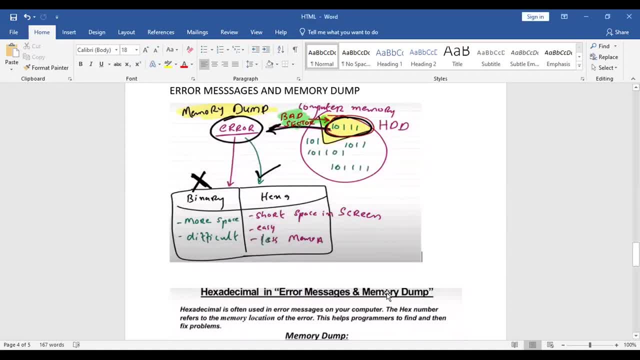 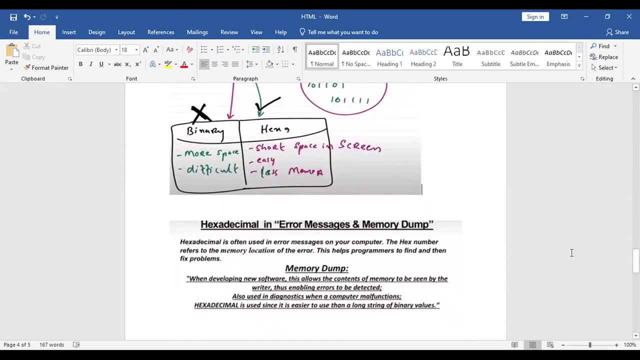 Now it is written here hexadecimal in error messages memory dump. So hexadecimal is often used in error messages. So this error message is on your computer: the hex number. the hex number tells us the memory location of the error. The memory location of the error tells us the hexadecimal and this helps the programmer. that here is the memory location of this error. it comes in hexadecimal and helps the programmer to go to this place and correct the problem. 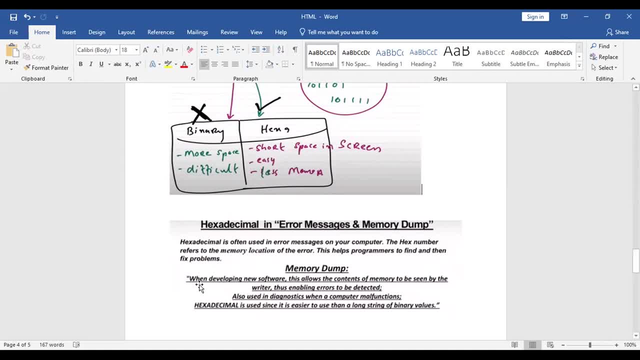 Now memory dump. when developing new software, this allows the contents of memory to be seen by the writer, thus enabling errors to be corrected. So this is the place where, when we are developing a new software, a program, then the contents of memory are seen at one place. that place is called memory dump. 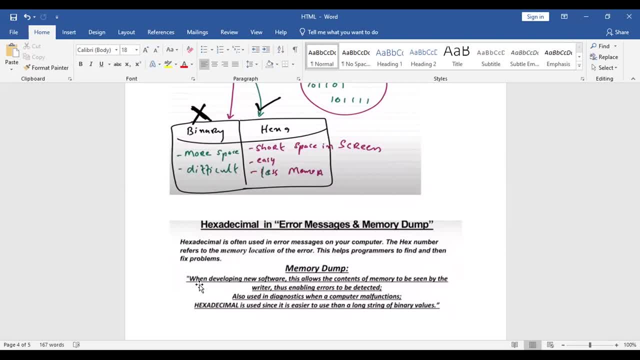 And the writer or programmer can go there and see that this is the problem, that I correct it before running the program so that this problem does not come next. Also used in diagnostics: I have used computer malfunction. if the computer is damaged, that is, if there is any problem in the computer, if there is any crash, then memory dump tells us that there is a mistake here. 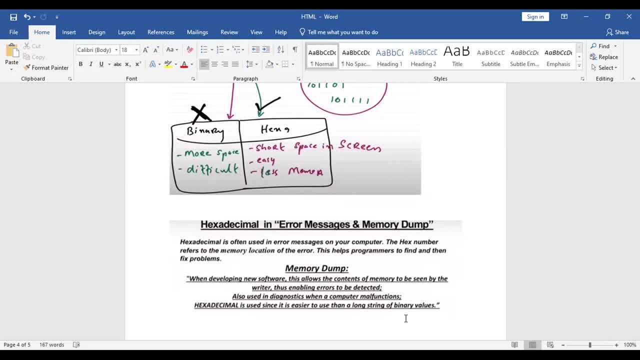 The hexadecimal is used since it is easier to use in a long string of binary values. So if it is binary, then it will be very big, In the same way we understand it by making it small. This error code is an indicator to a user of a piece of hardware or software that an error has occurred. 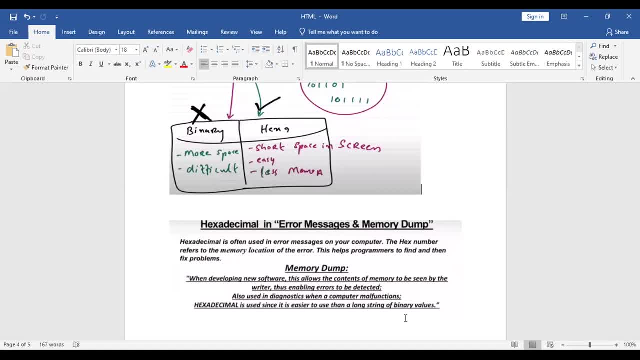 If there is any problem in the hardware or software, then it is an indicator that there is a problem here. This is numeric or alphanumeric code. This means that it is a hexadecimal code that determines What is the nature of the error. So why does memory dump come? 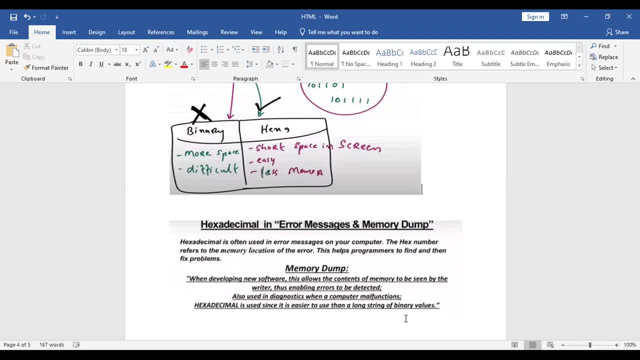 Memory dump may be that some system file has been corrupted, Some hard disk has been damaged, Sometimes RAM has been corrupted- Compatibility of hardware and software. So memory dump records all the content of the system, Like if the computer has crashed unexpectedly It has stopped. 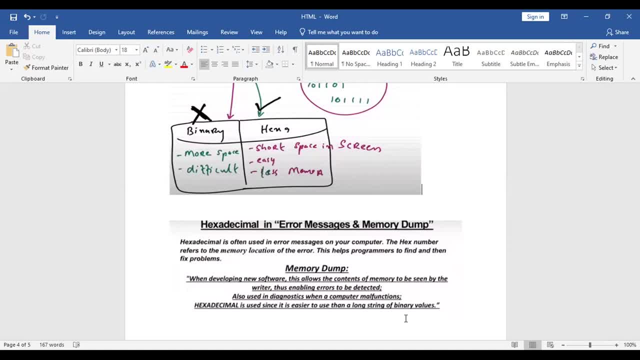 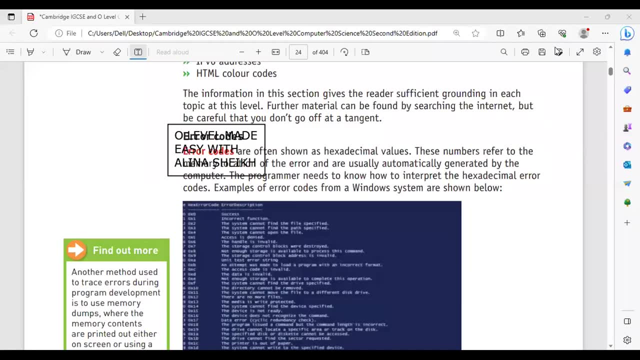 So it has recorded everything that was right before, then it happened, then it happened, So the person can go and see that this is the problem. Fix it like this. Now let's see ahead Here. you have given this example of this error code. 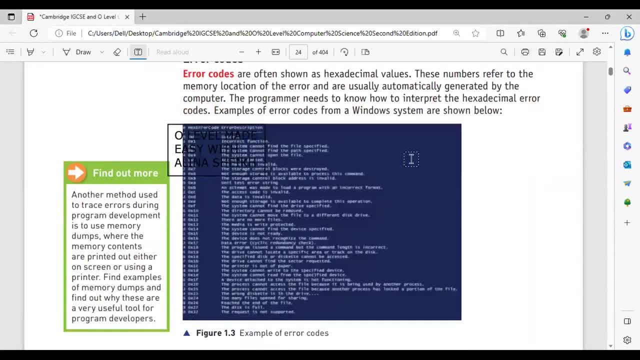 Here. you just have to look at one view that hexadecimal is also given to us. Here is the hex error code. Here 1F is written. Just go through the things written in this way And there is no need to pay much attention to this example. 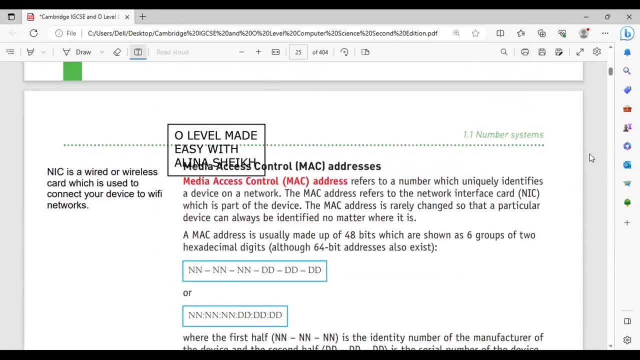 But what I have explained to you, you must have understood. Now, MAC address. MAC address is media access control And full form is its media access control. This MAC address refers to a number which uniquely identifies the device on the network. Means: I have a device. 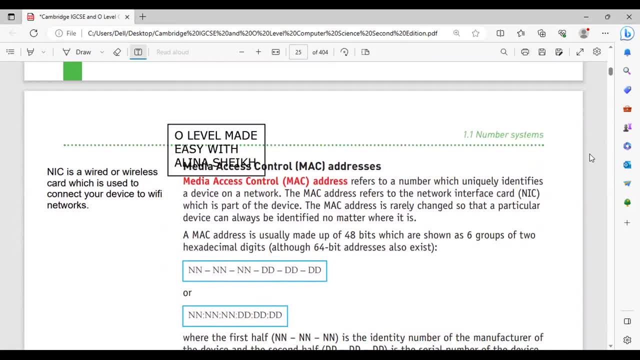 It has NIC in it. What is NIC? NIC is a wired or wireless card Which connects our device to Wi-Fi. Okay, The name of this NIC is MAC address. MAC address is also called physical address and hardware address. It is in our cell phone, laptop, tablet. 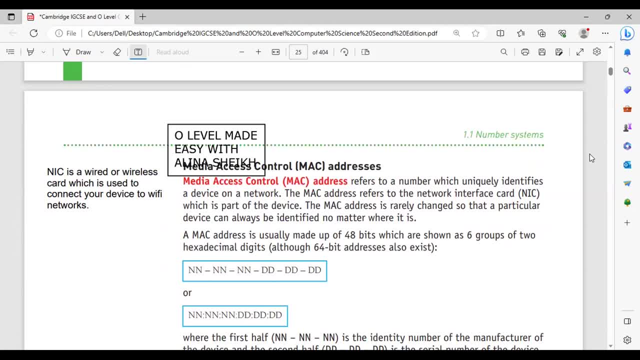 It is in all of them. It means every device has a name. Its name is in the form of number. I say its name is this. So it has given the number that this name is in the form of its number And every device is unique. 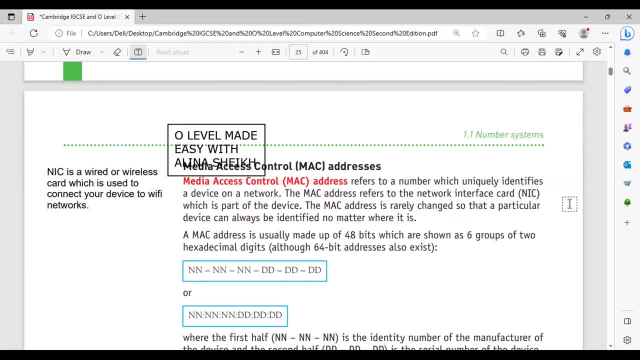 It is written uniquely Means every device has a different MAC address. MAC address refers to NIC, which is a part of the device. Here I have written its definition of NIC. I would strongly advise you to copy this with you. NIC is a wired or wireless card. 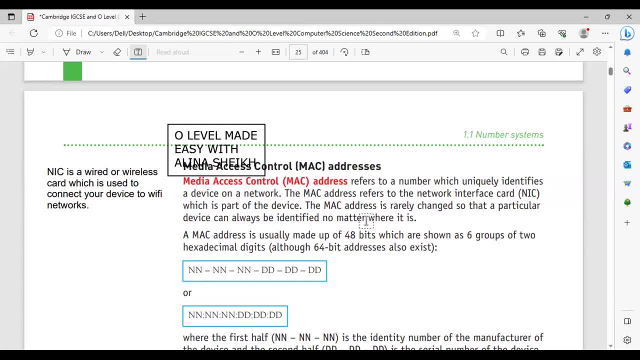 Which is used to connect your device to Wi-Fi network. After that, MAC address does not change, So that when the birth of the machine is made, MAC address is given to it And till it is destroyed its MAC address does not change. 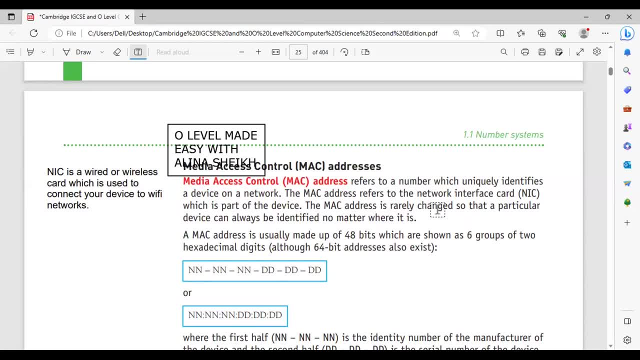 Okay, And MAC address does not change, even if it is somewhere, Because then it uniquely identifies where the device is. For example, we see in the movie that when a thief goes, he picks it up and throws his mobile somewhere else, Because he knows that the police will trace it. 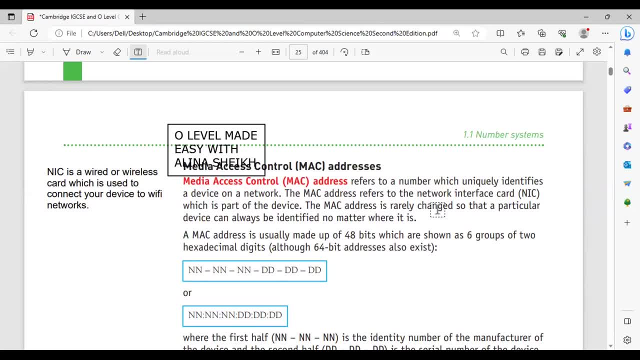 How will they trace it With MAC address? If a thief has stolen something, then he will have a MAC address with the police. When he has a MAC address with his mobile, then he will trace it through it Now instead of taking someone else. 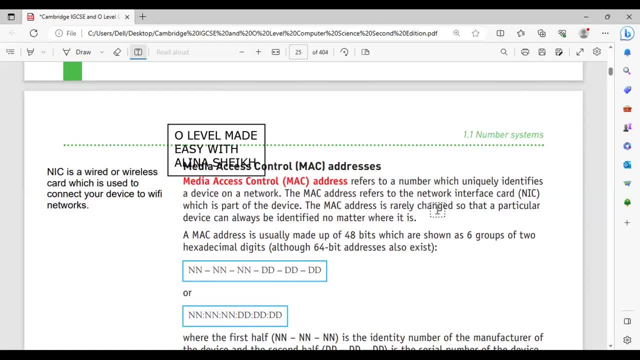 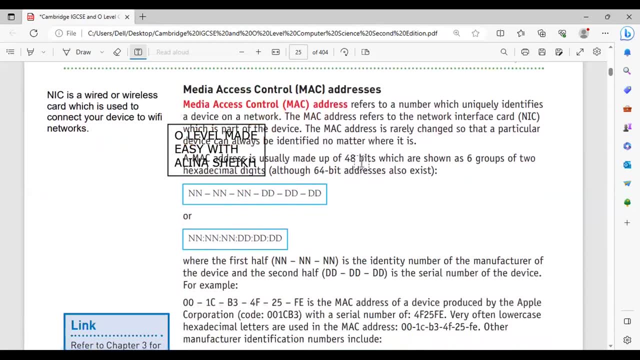 he will take the mobile with him. Why? Because there is a MAC address in the mobile. He will identify it by identifying where this device is. Okay, In this MAC address we can also have 48 bits And 64 bits. 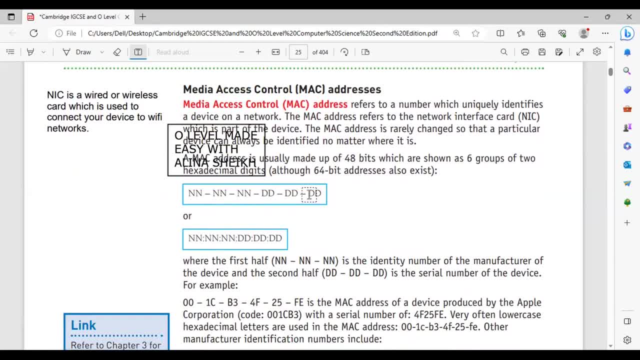 And 64 bits also exist And there are 2 hexadecimal digits And they are also of 6 groups. There are 6 groups and 2 hexadecimal digits. Either a dash comes here and a dot comes here in the middle. The first half is the identity number of the manufacturer. 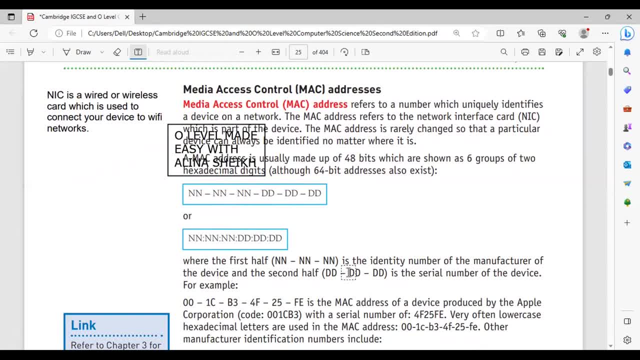 That is the organization that made it. The second half is the serial number. Like the serial number, there are a lot of mobiles made, So they give the serial number. This is the first, this is the second, this is the third. 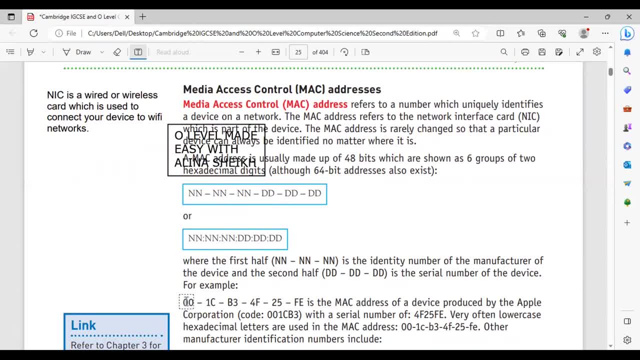 This is what Apple made: a device. So he kept his MAC address here. This is the manufacturer number of Apple, The identity number of the manufacturer. All the devices of Apple will be from him. And 4F25FE. This will be the serial number. 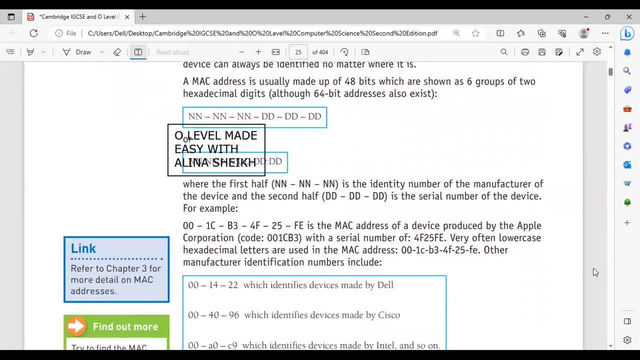 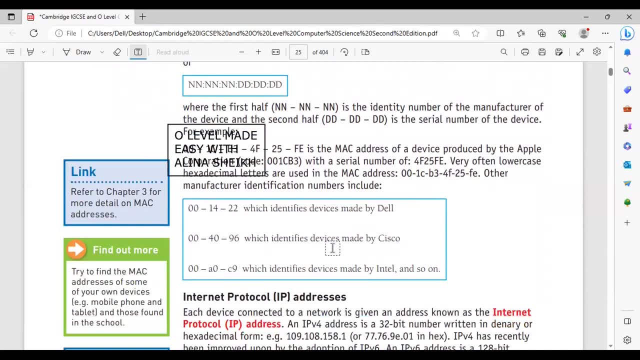 Now lower case is also used And upper case can also be used. No worries, These are the devices that will be made from our Dell. That is 001422.. Cisco made it 004096.. Intel made it 00A0C9.. 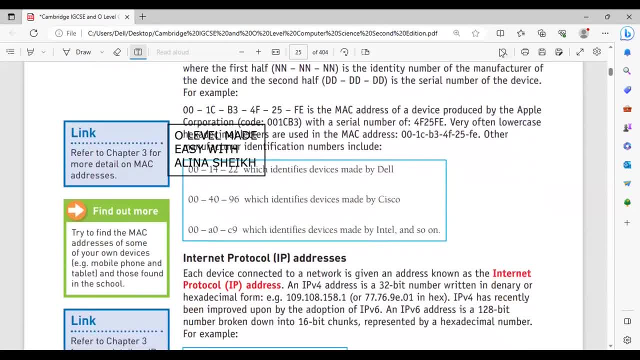 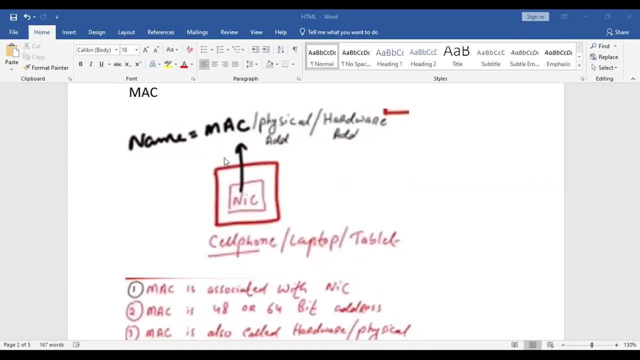 So in this way, Each C has a different logo. Now let's understand it more. Let's see through the diagram. Now, this is NIC. Its name is MAC. MAC is also called physical address, Hardware address is also called Cell phone, laptop, tablet, etc. 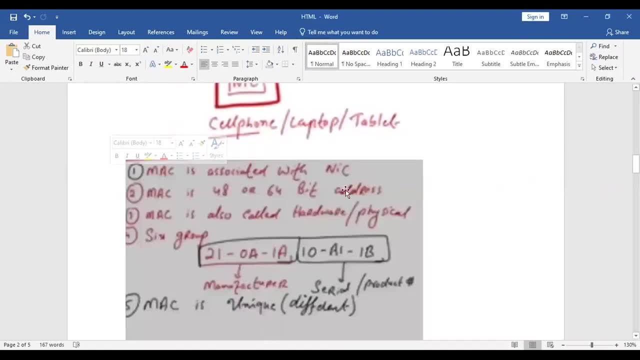 It is in all of these. Now what is this? MAC is associated with NIC. It is 38 and 64.. I have made pointers here So that you can understand easily. Hardware physical address is also called. There are six groups. 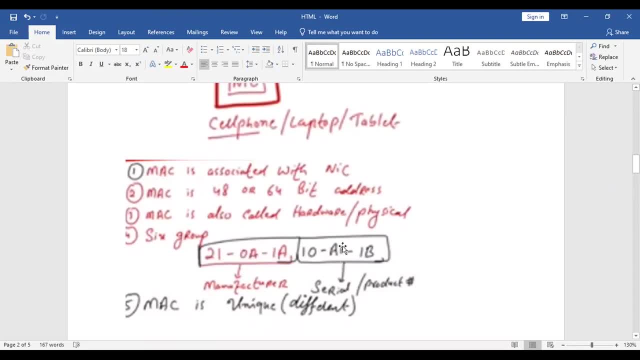 There are six groups and two hexadecimal digits, Meaning there are six groups and two hexadecimal digits are made. First is our manufacturer, The number of the manufacturer is that, And then the second serial is the product number, And MAC is unique for everyone. 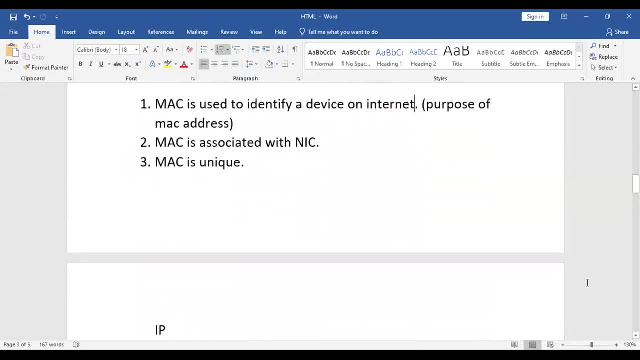 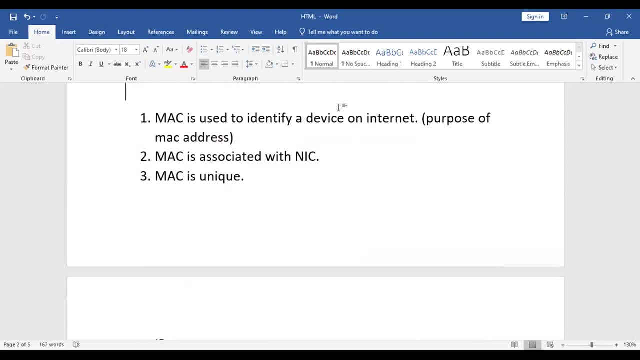 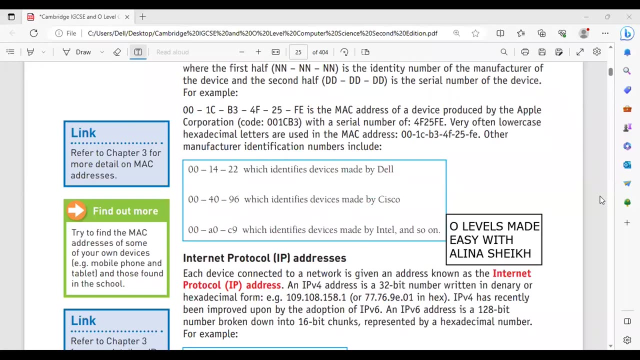 It is different. MAC is used to identify devices of the network, If asked what is its purpose. So MAC identifies a device on the internet And it is associated with NIC, And MAC is unique. We have IP address. Any device that is connected to the internet has an IP address. 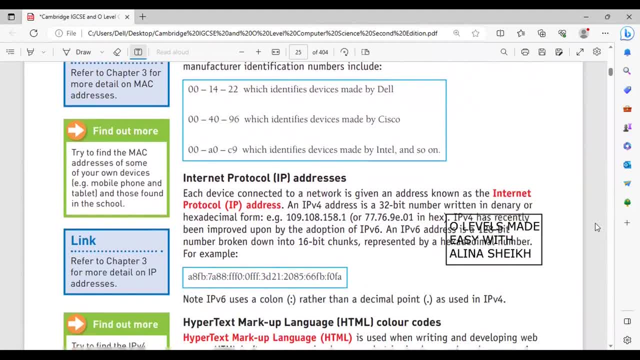 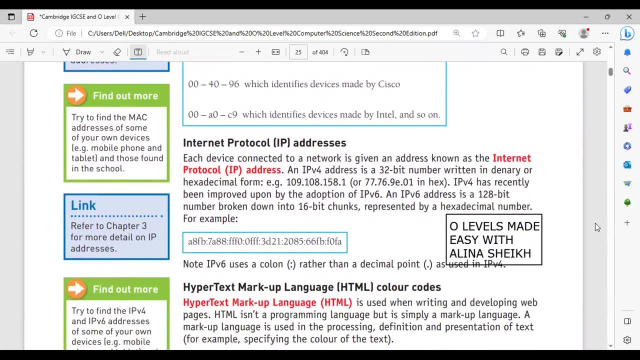 IPv4 and IPv6.. What is IP? Its full form is internet protocol, So the internet protocol is with every device that is connected to the internet. IP address is a unique address that identifies a device on the internet or local network. Now the internet protocol is its full form. 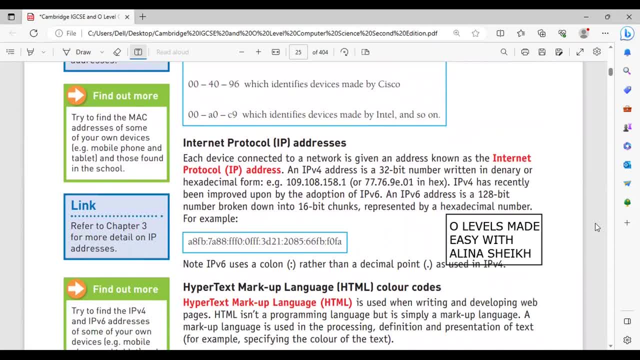 What is internet protocol? It is a set of rules governing the format of data sent via internet or local network. It identifies a hardware device on a network. Now here we have two types of IPs: One is the old version and the other is the new one. 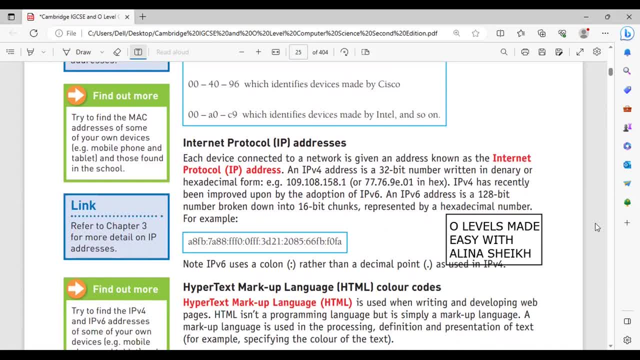 One is IPv4, the old version that we are using till now. I have IPv4.. The new one is IPv6.. It is very rarely used, But it is a future generation, Meaning of the next generation. It is a technology. 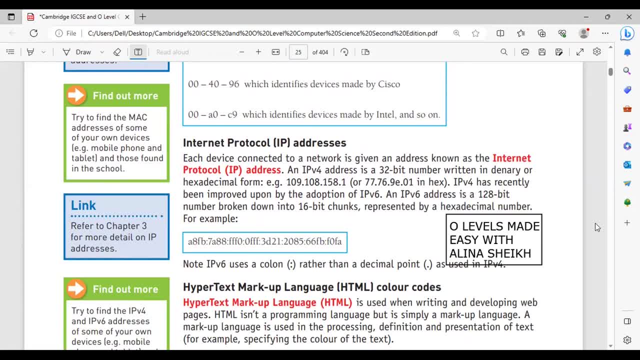 So IPv4 is a 32-bit number Which is written in DINUI. It is in hexadecimal form. How is IPv4 improved Through IPv6.. IPv6 is a 128-bit number. It is broken into 16-bit chunks. 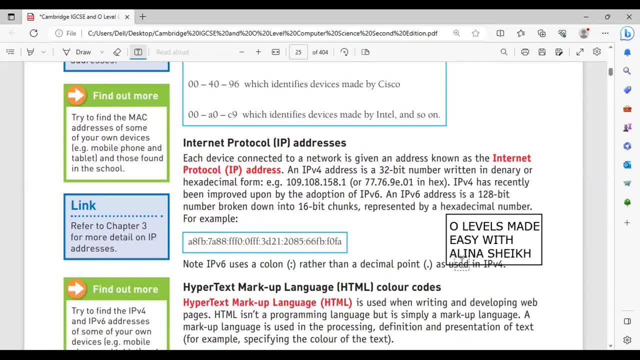 And it is represented through hexadecimal number. IPv4 uses decimal point And IPv6 is a colon. Now look at this and tell me: Is it IPv4 or IPv6?? Obviously it is IPv6.. Why? Because a colon is being used here. 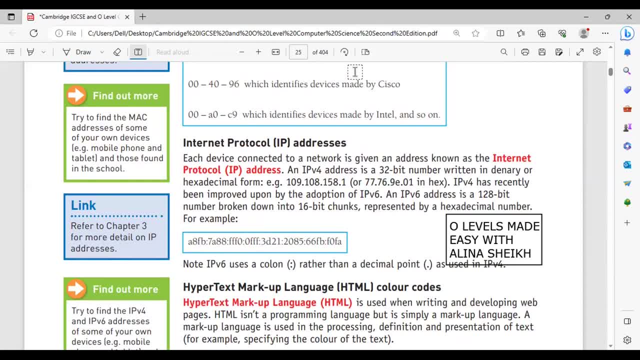 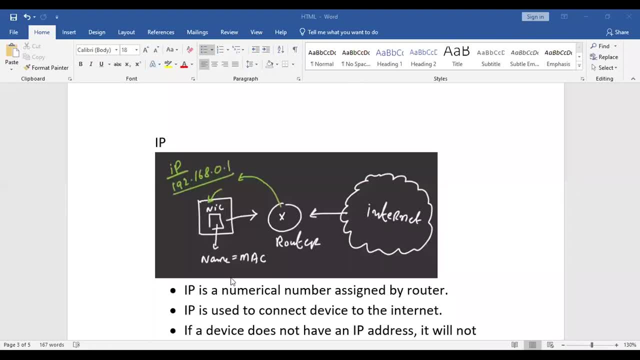 Instead of the decimal point. The IPv4 used to be a decimal point. Now we will see it in more detail. Now. look at this. This is my device. Its name is Mac. Whatever its name is, It is a Mac address. 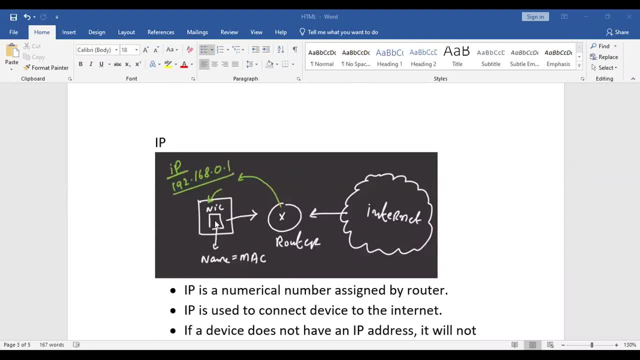 It is a number. It belongs to that device. It is its home. Okay Now, whenever I want to connect to the internet, My router will assign me an IP. IP is the number that will connect me to the internet. I will not go to the internet until I have IP. 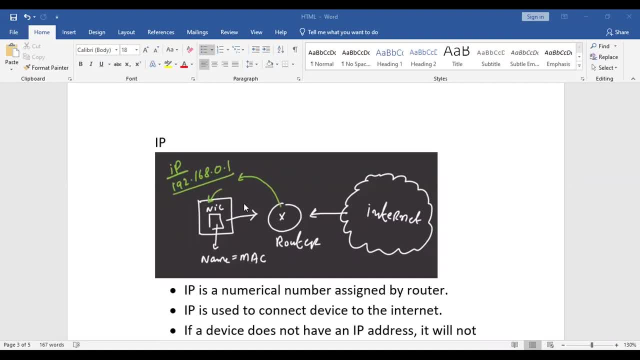 Router told me that this is your IP. You are going to the internet with this name And whoever is there will recognize you with this name. Okay, This means that this is an IP. This is a device that this device is using, So the router gave it to me. 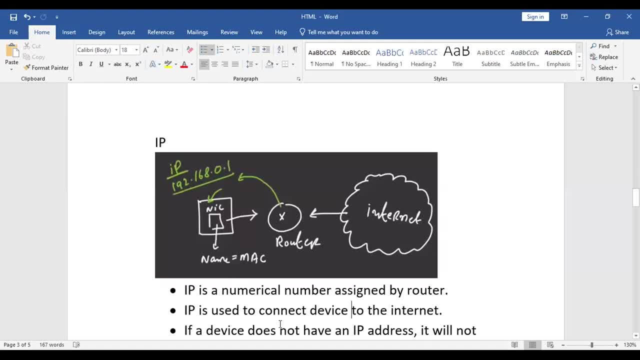 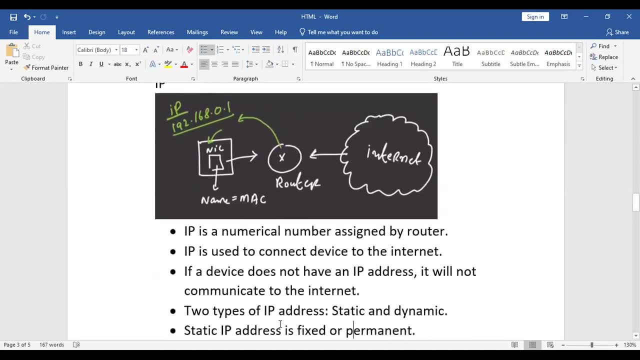 So that people know that this is the device. Its IP is this: IP is a numerical number that the router has assigned. IP will connect the device to the internet. If a device does not have an IP address, Then it will not communicate with the internet. 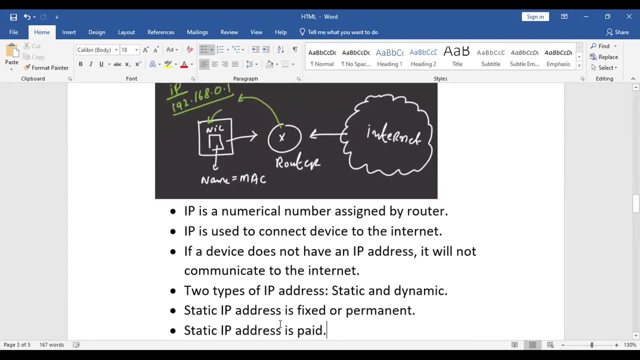 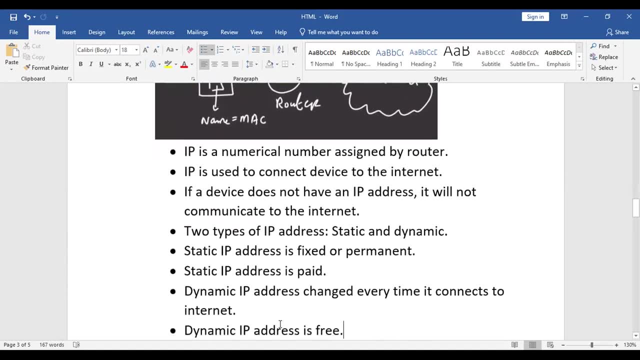 There are two types of IP. One is static, One is dynamic. We know that static means fixed, So it is fixed or permanent And it is paid. Dynamic IP address changes every time when it connects with the internet. And dynamic IP address is free. 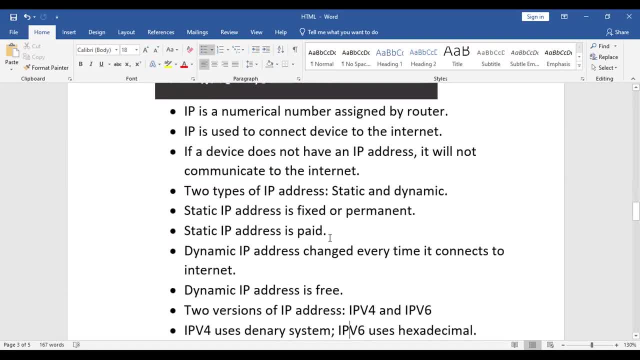 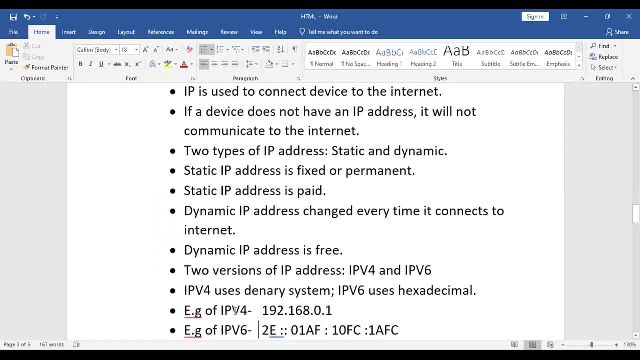 There are two versions of the IP address. These two types- static and dynamic- And two versions of the IP address: IPv4 and IPv6.. IPv4 uses the binary system, But IPv6 uses the hexadecimal. For example, 192.168.0.1 of IPv4.. 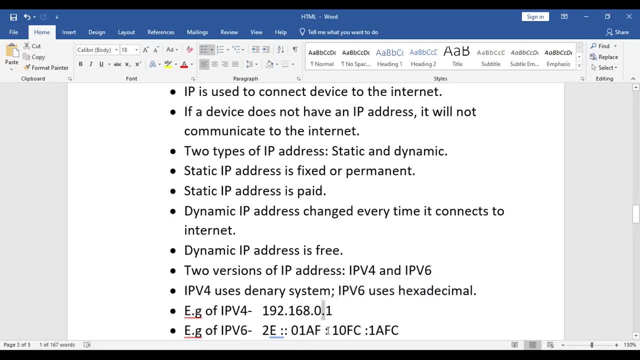 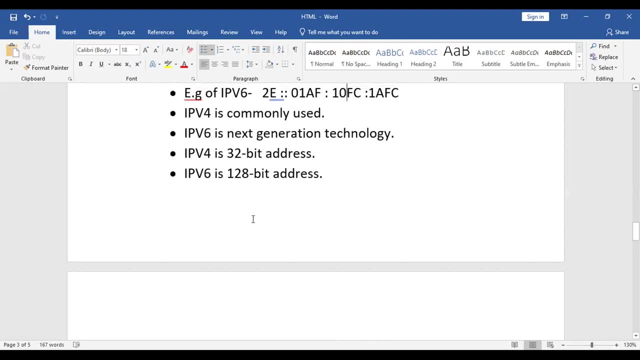 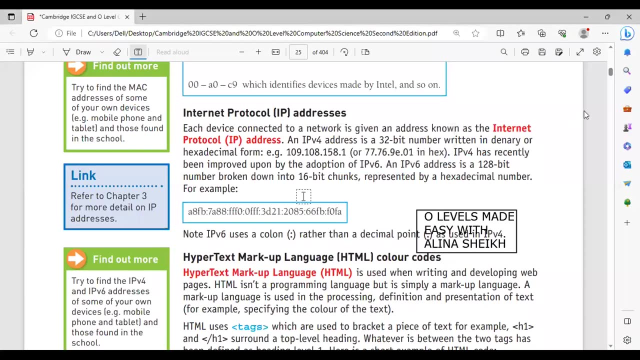 The dot. here is the decimal point, and if IPv6 is here, then colon is used. IPv4 is commonly used. IPv6 is next-generation technology. IPv4 is a 32-bit address and IPv6 is a 128-bit address. Now let's come to HTML. How many uses have we done? Let's see how many we have done so far. 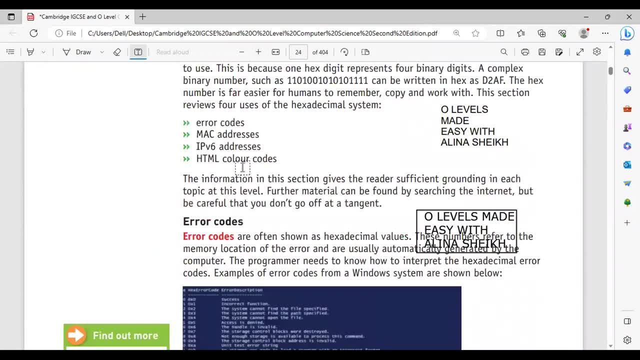 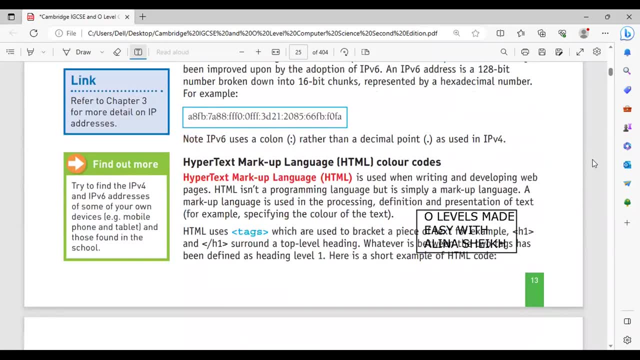 We have error codes, MAC address, IPv6, HTML color codes. the scene is done now. there is only one last. Now, the last is HTML color codes. What is HTML? It is a hypertext markup language and it is used when we write, write or develop a web page. 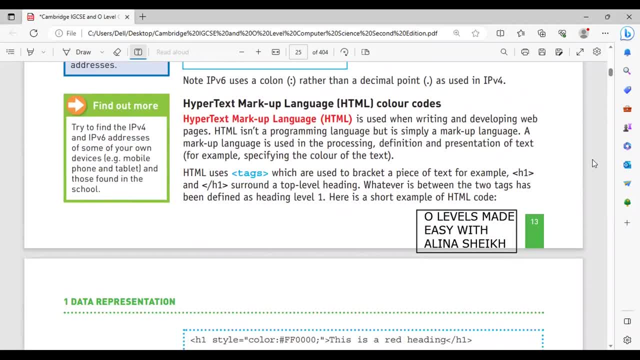 It is not a programming language, but it is a markup language. To run the programming language, it needs a translator from the back. But markup language is not a markup language. So HTML is a markup language. Markup language is like makeup. In the same way, HTML is a markup language that makes up the entire web page where we use it. 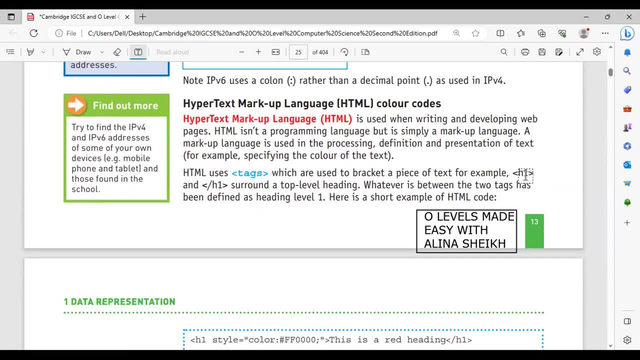 Now we will read this. When we write something in HTML, it is inside the bracket tag. We will write whatever tag is inside it. This will surround it. When we start, we have to open the tag, Write it in this way. 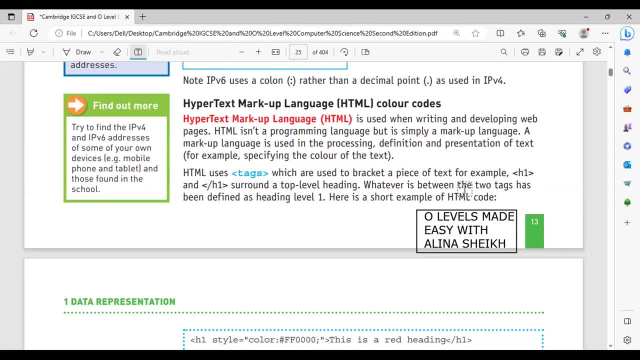 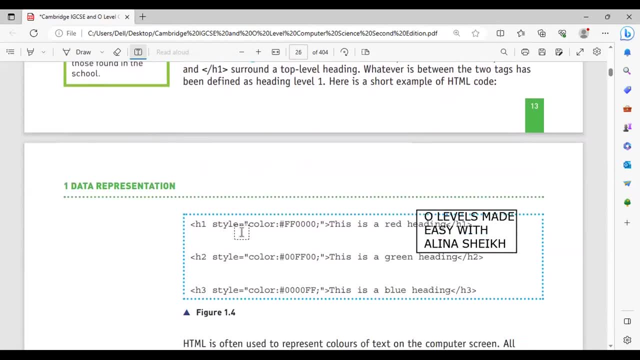 When we close it, there is a slash. Let's end that tag. Whatever is in the middle of that tag, then the heading will be 1.. Now let's see a short example of this. What is this? H1 style. 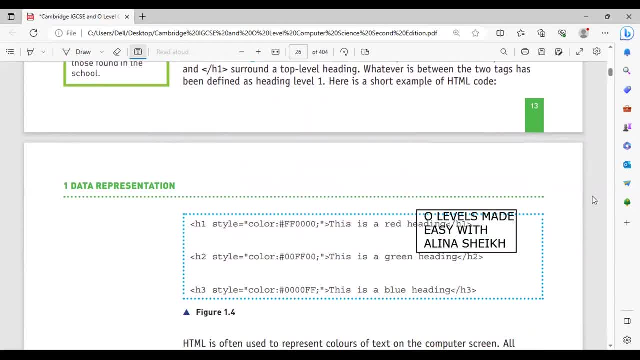 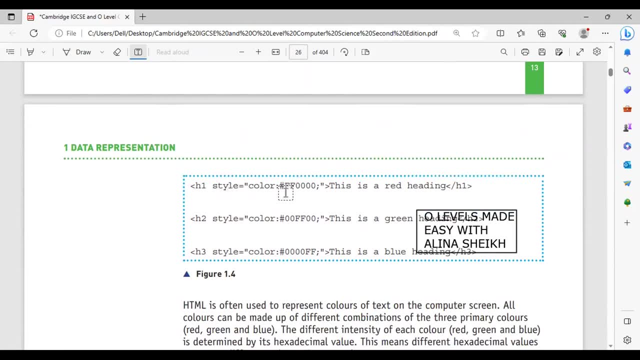 Here it started. and then I wrote as equal to color. You don't have to go into so much detail, But still let's read the same thing, H1 style. Then I wrote the color. Here is the hash. We will read further: 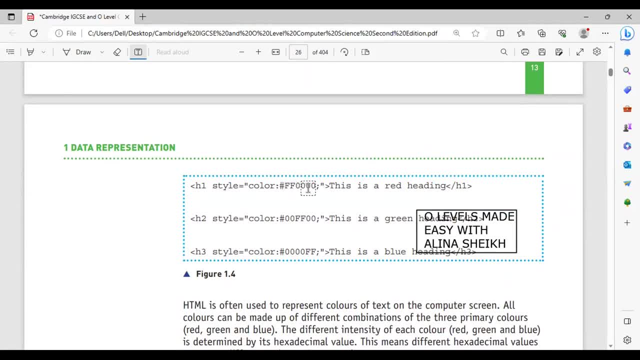 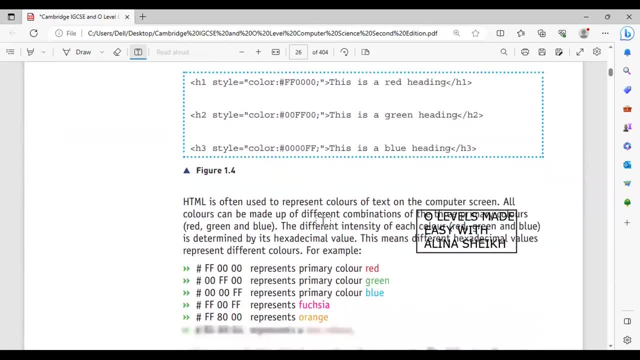 It will come now. Then after that, I told the color here and then I wrote: this is a red heading, And then when I want to end the tag, it has a slash, In the same way it happened here as well. Now, HTML was not a programming language. 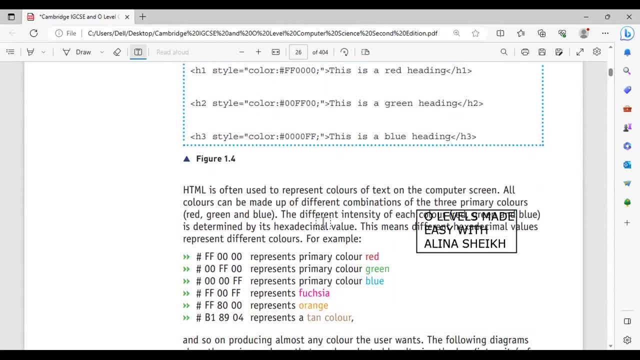 It was a markup language And it creates, develops and authors web pages. Whenever we write HTML, we write it on a notepad. When we write on the notepad, then when we save it, we write html. Next time we open it it will open in Google with you. 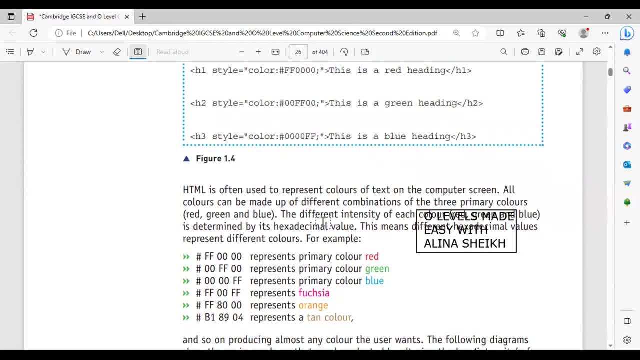 And who translates it? Browser translates it: Browser? what is it? Google, etc. Mozilla- all these are browsers. Browser is an application program that provides a way to look at and then interact with all the information on the World Wide Web. 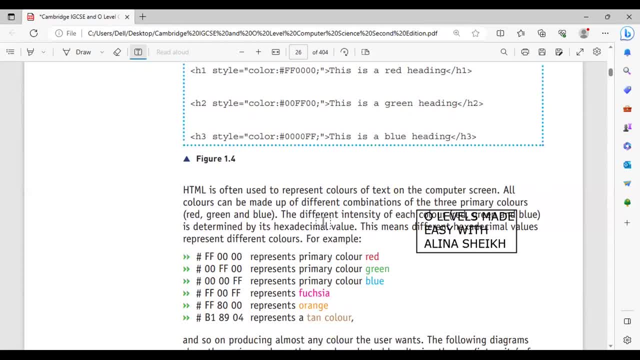 That is, we interact with others. Okay, We wrote the program in HTML through notepad. Then we wrote: save as html, So the web browser will translate it. Then we will go to the web page and we will get its preview. 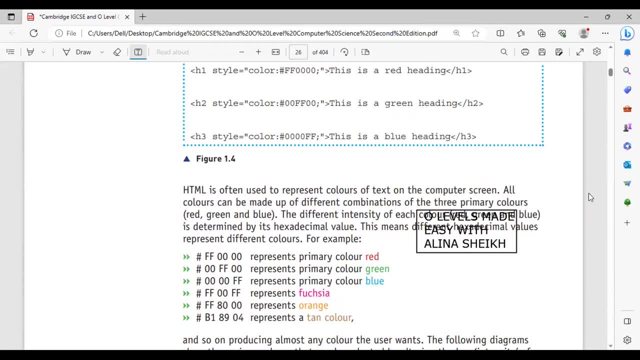 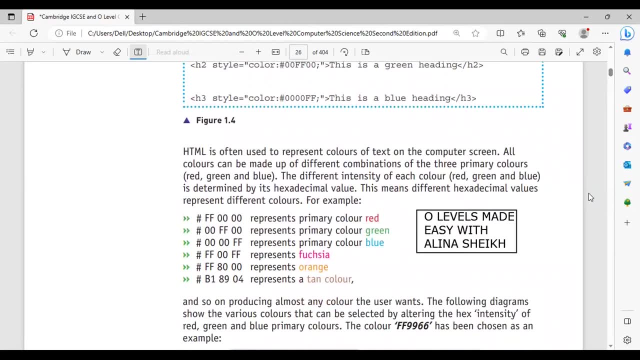 HTML is then. Then we also represent the colors on the color screen. All the colors are made up of three primary colors. What are they made of? R, R, G, G, B, B, How? Let's see now. 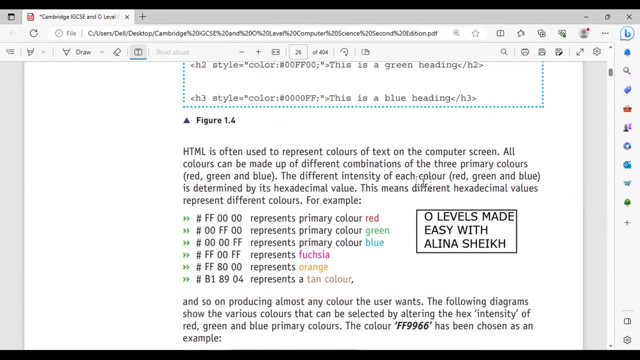 There is a different intensity of different colors. Which are these three primary colors? Red, green and blue. These three colors are made up of different colors by mixing them. Now, these three have different hexadecimal values. This means that the different hexadecimal value of these three is determined. 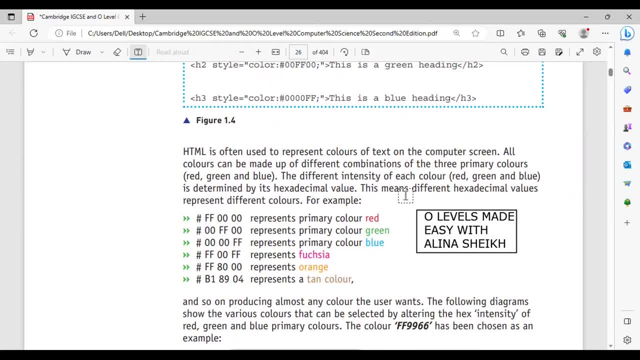 This means that different colors will be made up of different hexadecimal values, Like 0 till F. The hexadecimal value is 16. 0 till F. So we have three colors: Red, green and blue are determined by hexadecimal values. Different hexadecimal values represent different colors. 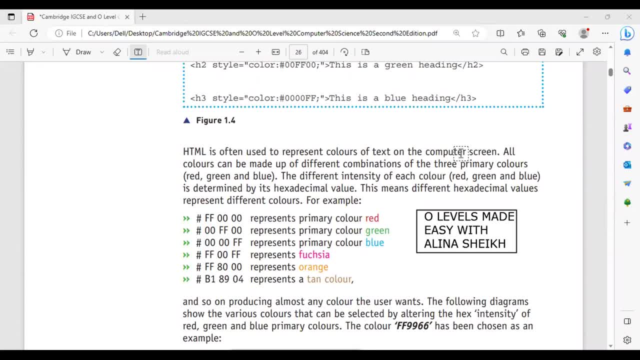 0 till F is our hexadecimal. 0 till F is our hexadecimal, So 16.. Base is 16.. So it means that if the intensity is less than 0 till F, then the color will be 0. If it is more than 60, then it will be F. 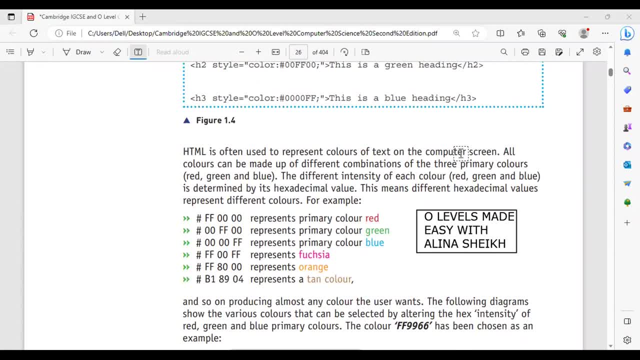 or it will be F. In the middle of this we have 1,, 2,, 4,, 5,, 6,, 7,, 8,, 9,, 10, well, it won't be 9 till 10, it will be A, B, C, D, E, F. 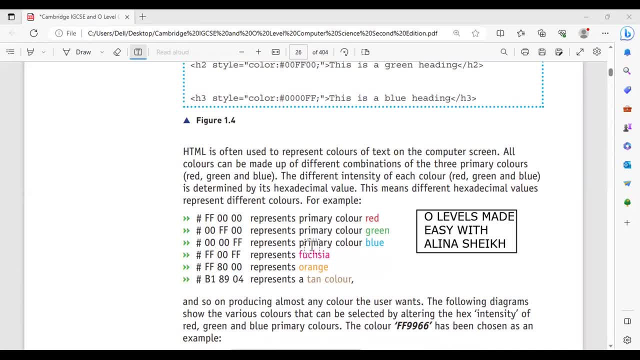 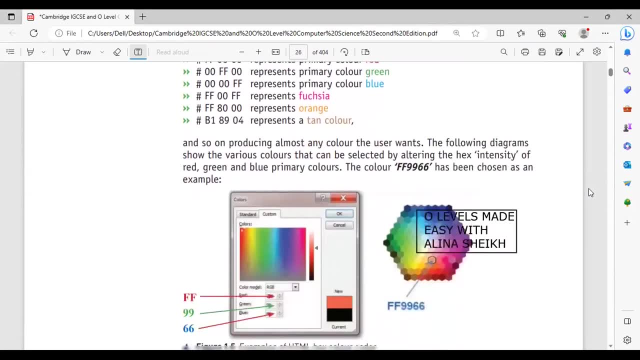 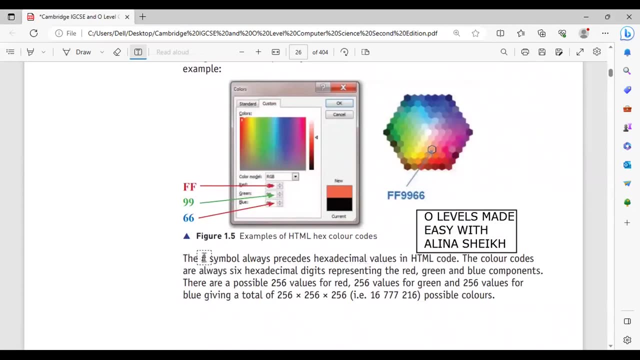 Now let's see it. Let me show you one more time. For this example, we have R and G. The first thing to see is that here there are different intensity types of colors. Whenever we write hexadecimal values in HTML code or we make the color represented, 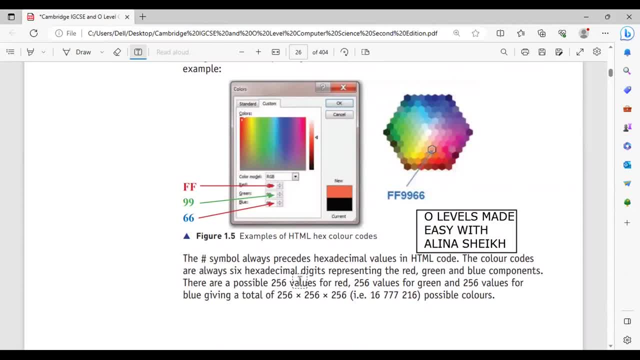 the sign of hash is required. The color codes are always six decimal digits. Red, green and blue components are told Now red has 256 values, green has 256 values and similarly, blue has 256 values because it is 0 to left. 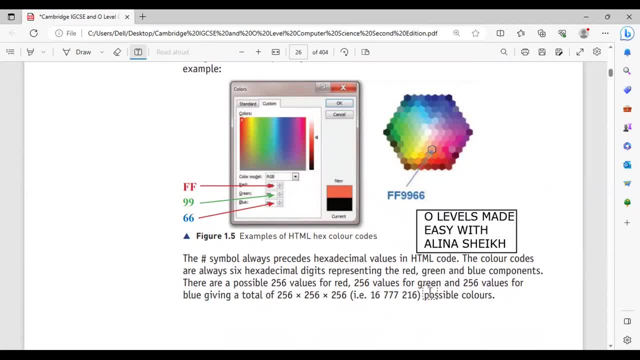 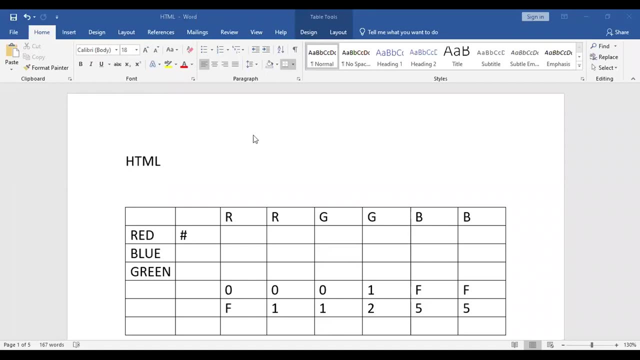 So everyone has 256 values. So when we multiply 256, 256, 256 by all three colors, then we get 16.5 million different colors. Now let's see it one more time. This is our HTML. I have designed one thing for you. now see. 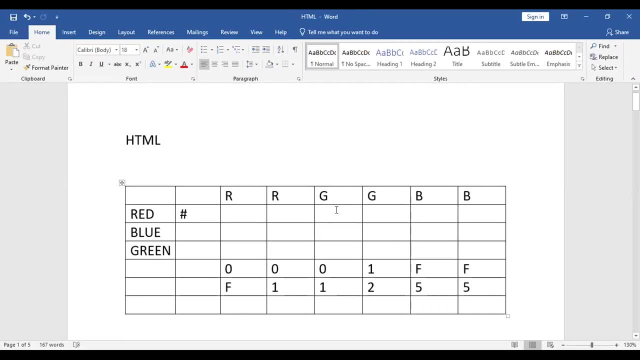 Hashtag sign has come: RRGGBB. I said RRGGBB, only these three are there. Whenever you were told to make red color, I said: I want pure red, I want red only. So what I have to do is I have made full intensity red FF and rest 0 is applied to it. 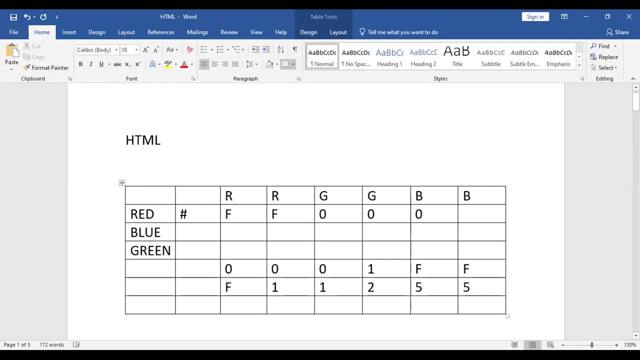 0 green and 0 blue means I got red. Now, similarly, if I want blue, then I first put the hashtag sign. I said not red, I want only blue, So I made rest 0 and full intensity means I gave blue on F. 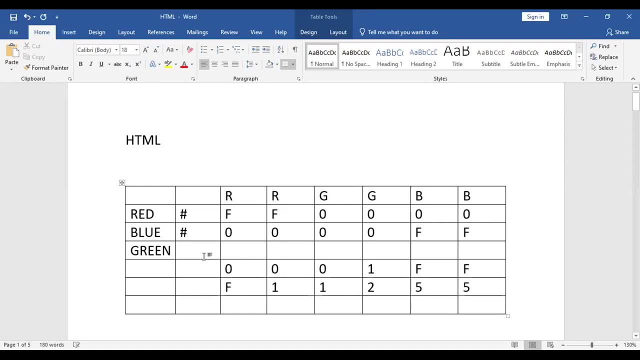 After that I said: now I want green. sorry, here is green. Now I said: I don't want red, I don't want at all, I want full green. I gave FF, that is, I gave full intensity. Now, if I tell you that I have written this number below: 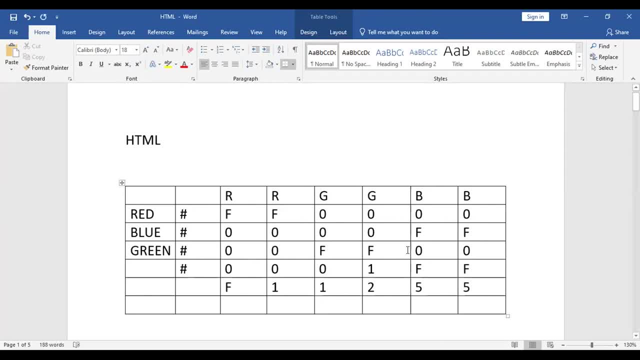 on hexadecimal number, you tell me whose shade will come. whose shade is it? Red is completely closed. green is also almost closed. after 0, it is closed. there is no special intensity for it: 0,, 1,, 2, it will keep going like this, and F is also very intense. so this is shade of blue. 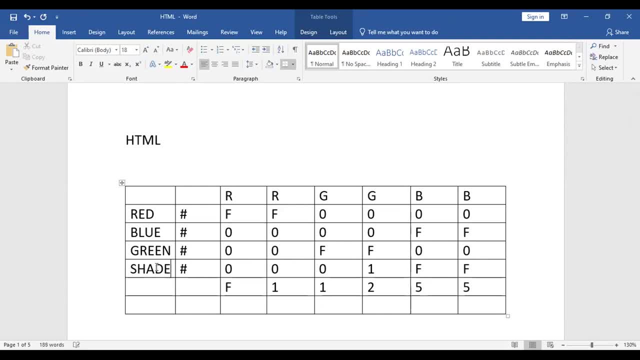 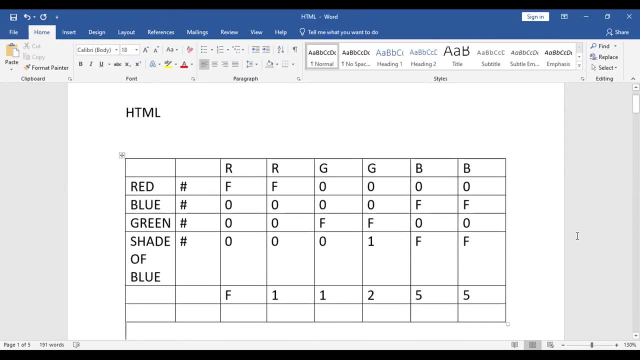 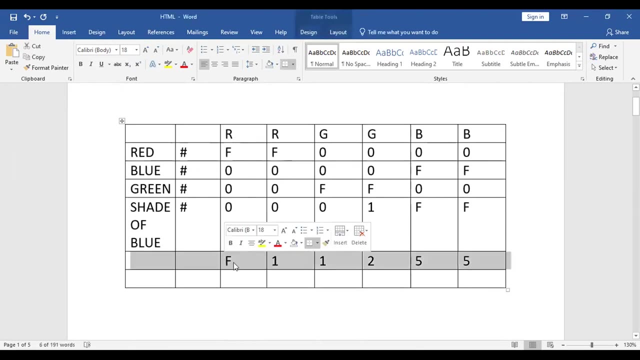 means it is almost giving us blue, so I can say that this is shade of blue. after that, if I say one more number, what is that? If I say F, 1,, 1,, this number, so red is F, means there is F on red, so it has full intensity. and then G is 1,, G is 2,. 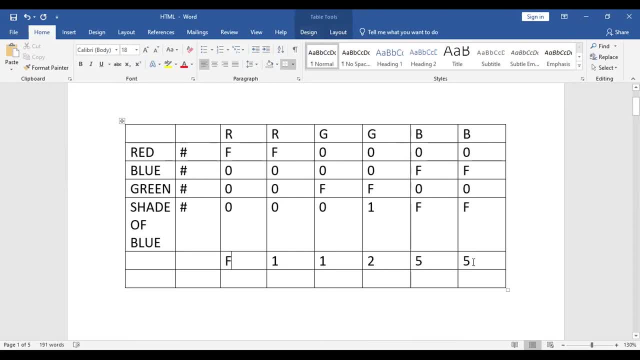 means it doesn't have much value. 5,, 5, it is very less. red is very intense, so whose shade will come? This is shade of red. let's make another color and see: okay, yellow, if I said. 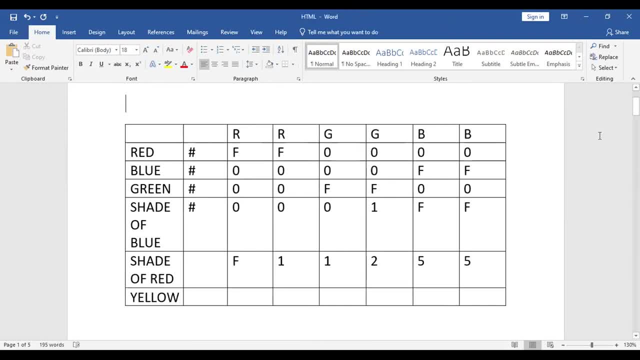 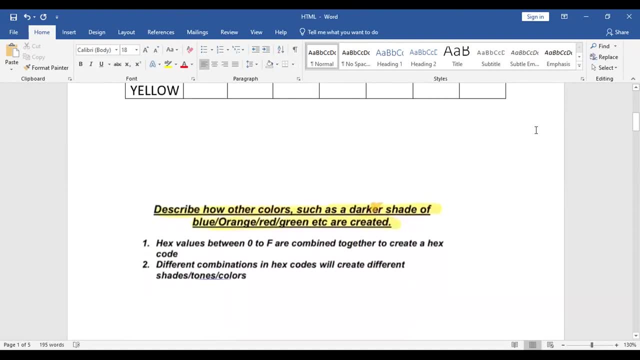 so we do this. I have out it a question of pass paper. we see yellow there. it is attached to it. okay, let's come down. there is a question of pass paper. describe how other colors, such as darker shade of blue, orange, red and green, are created. 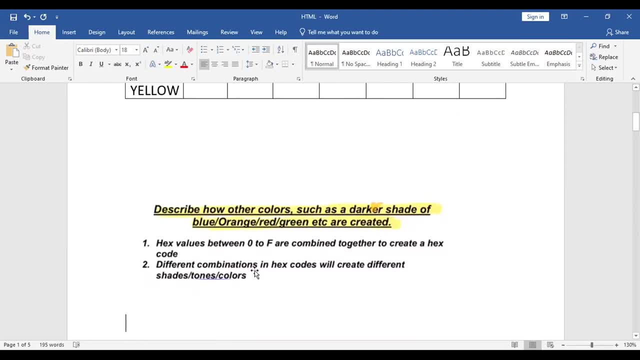 Now there is a question in your pass paper on which I wrote below. it was 2 marks, so it has to write 2 points. so how are the other colors? he said that in one color it becomes. but how are the other colors? formed different shades of them? 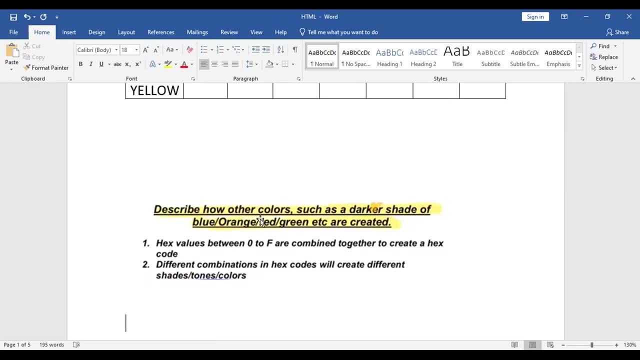 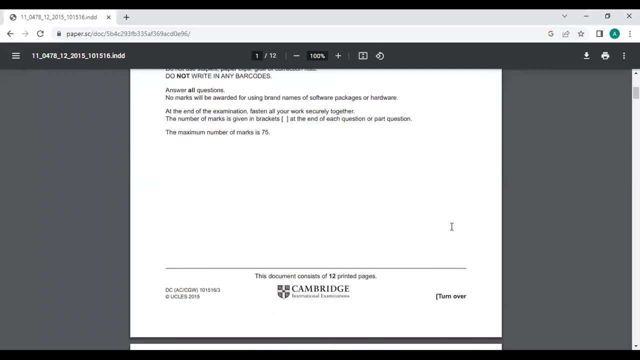 the hex values 0 to f. that combined, then they make the hex code. after that There are different combinations of hex code which will create different shades, tones and colors. Let's see one more fast paper question. Let's see the fast paper question from October-November 2015.. 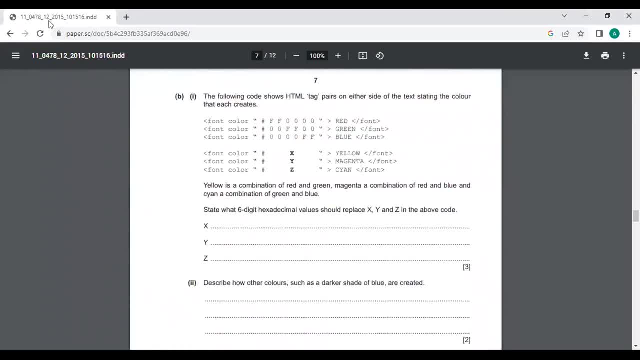 Now let's come here. There was a fast paper question, Let's see it. The following code shows HTML factors on either side of the text, starting stating the color. Here it is written that it is red, green, RR, GG and BB. 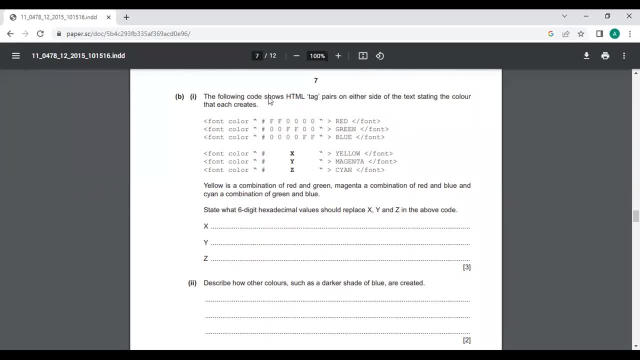 Now I will write it on top of it so that you can understand it easily. I wrote R on top of it, Then I wrote R on top of it, Then I wrote G on top of it, Then G on top of it, Then B on top of it. 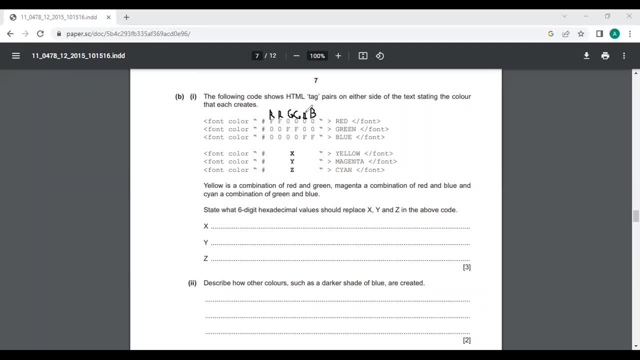 Now we have RR, GG and BB. Let's see: This is R, It is on top of it. It is F and F It is red on top of it. Then here is green on top of it And here is blue on top of it. 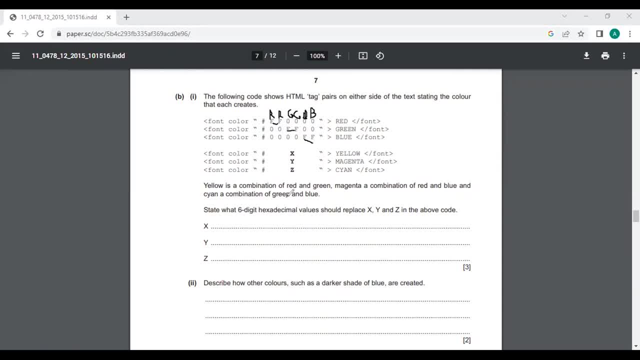 Here. I said that I want yellow, magenta and cyan. Now we don't need to remember what it is. I told you that yellow is a combination of red and green, And magenta is a combination of red and blue, And cyan is a combination of green and blue. 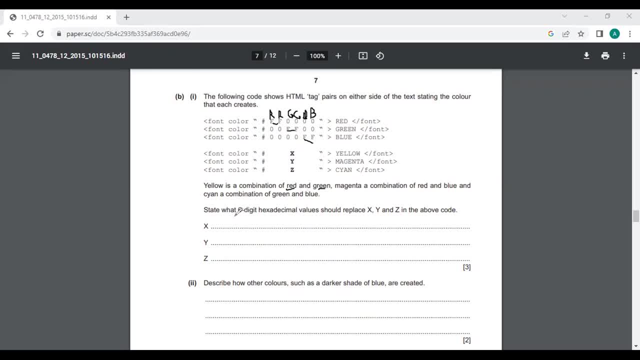 If I say yellowX, I will write 6x, x and x, But along with that I will write hash, x and x, And I will definitely write hash as well. I will do it correctly once. I will write it now. 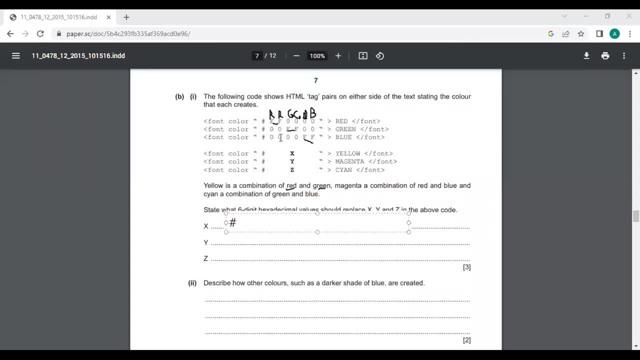 I wrote hash. Now yellow is a mixture of red and green, So I have RR. I opened R on full intensity, Then it is GG, It is red and green, so I opened it completely And the rest, blue, is not at all. 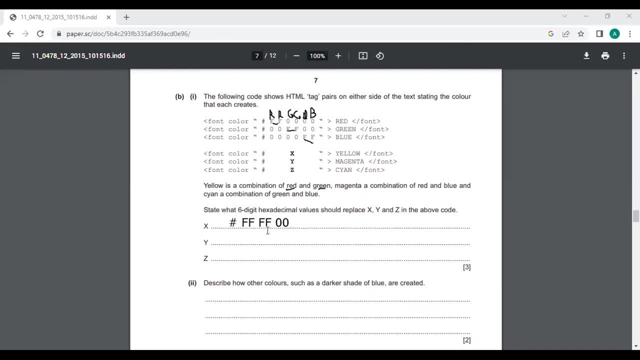 So I put zero on it. Then next, magenta is a combination of red and blue. So red and blue. First I have to put the hashtag sign. Now what is red and blue? So R, R means R, R, Then after that, G, G, G, So it is absolutely zero. And baby F, F. 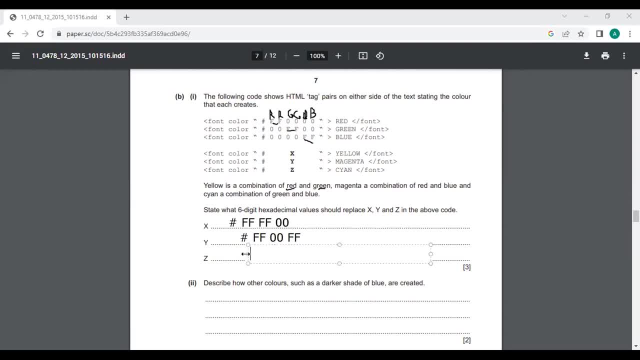 After that, this is green and blue combination, So red will be absolutely zero. The rest will come. I did zero, Then I did it F F, Then I did it F? F. So this is how our answer came. 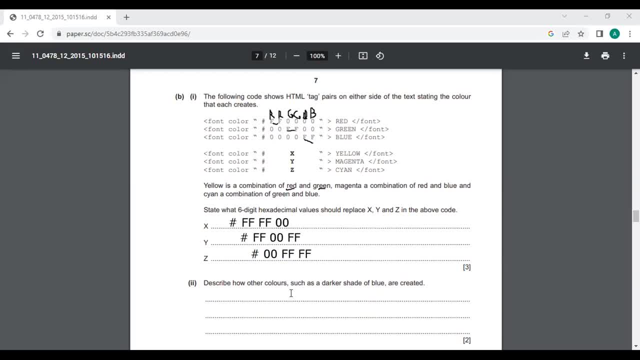 Now how are the other shades created? Are they dark or blue? We have just seen that hexadecimal is a chord. Through that hexadecimal is different. We represent it through hexadecimal. So when there is a different hexadecimal, then we give different combinations.